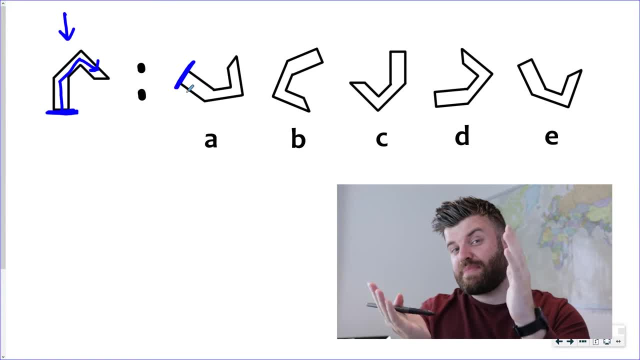 would be here A bit of an awkward angle, but if we rotated the paper- or in this case I'll rotate my head to have a look- Hopefully you can see how here's the base and actually the overhang goes to the left, So it can't be A. that's been mirrored Our shape overhangs. 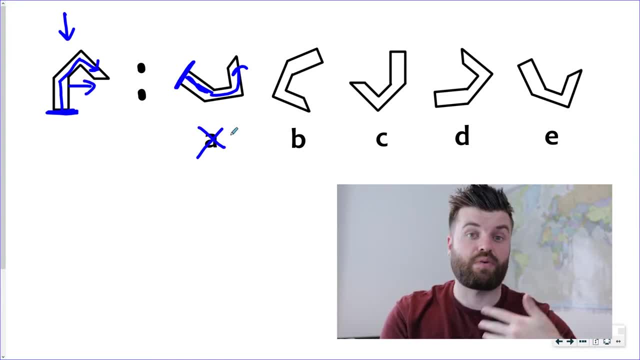 to the right. So we're going to use that technique now to go through the rest quite quickly. Let's take a look here. Our base is now there and it overhangs to the left of the base. That's not our shape. Look at this one now in the middle C. Now this one's upside down. 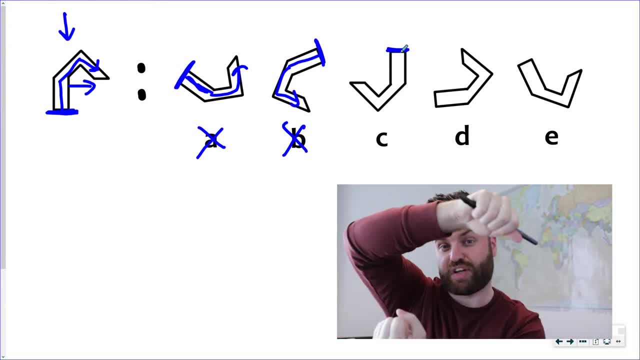 So I can't move my head upside down, but you'd have the paper and you'd shove it right around just like that to make it really easy for yourself. But what you should notice, with this shape, the base actually does go to the right for the overhang. So C is the answer. 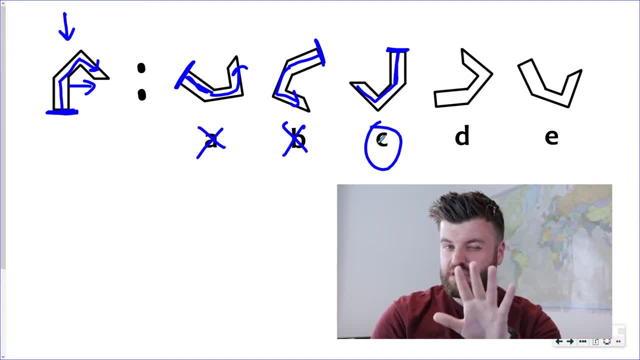 Now in the paper you can write down C and move on. but I'm just going to prove that the other two don't work. Here's D's base and it overhangs to the left. doesn't match up. And there's E's base and that one also overhangs to the left. 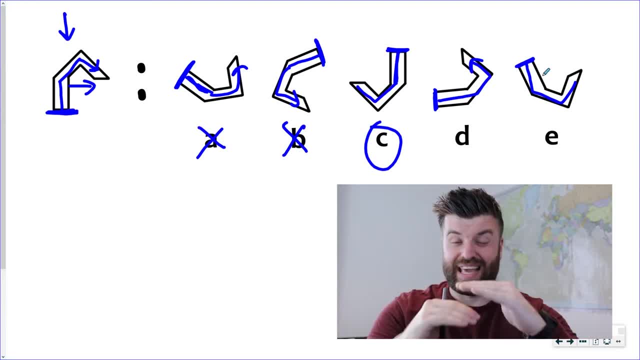 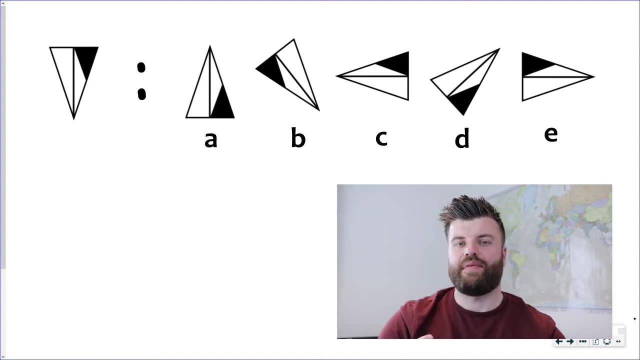 So rule number one for tackling these question types is: find a base for your shape, get something to work from, ie right or left, pick a feature of the shape and then try and match it up. Okay, let's take a look at another question Now. spatial reasoning can be tricky. The idea 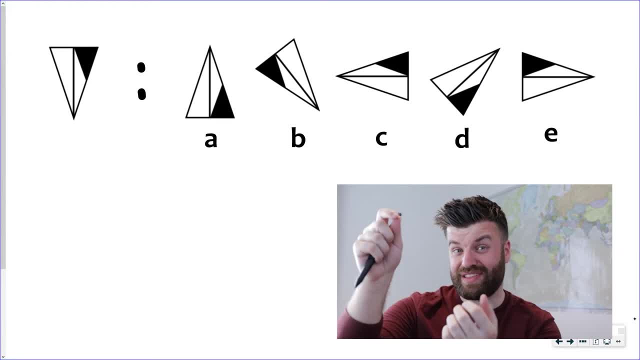 of these questions is for you to use your mind's eye and imagine that shape moving. Now, of course, you can move your paper, as I mentioned before, but just start to practice rotating that shape in your mind. Let's do it now with the shape on the left. Imagine that triangle. Let's look at the features. 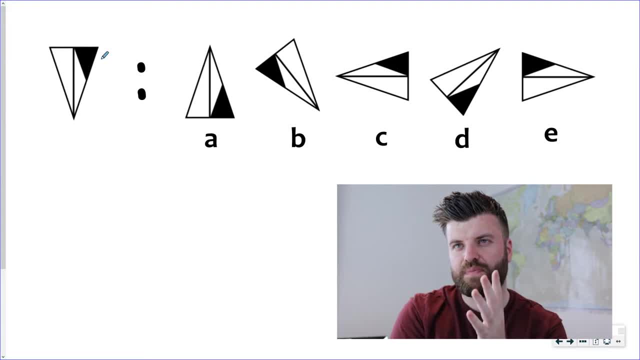 We've got a black shaded bit in the top right. We've got a line down the middle. Now just imagine this shape starts to rotate. Imagine it rotates 180 degrees. Would that black area here still be on the right hand of the shape? It wouldn't. It would have rotated around. 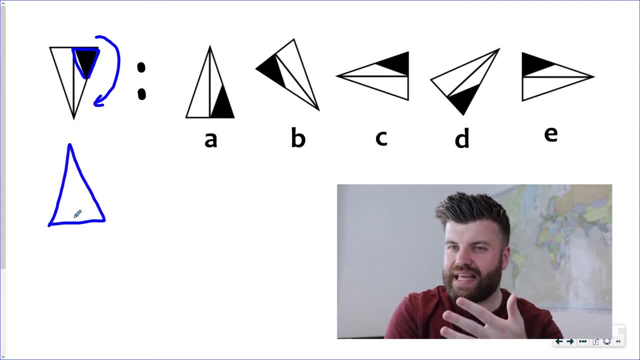 to the bottom left. So hopefully, just getting that practice in, you can start to draw to practice what the shape might look like. It would actually look something like that, So that on the screen now doing that the start might again help you when you're finding the shape on. 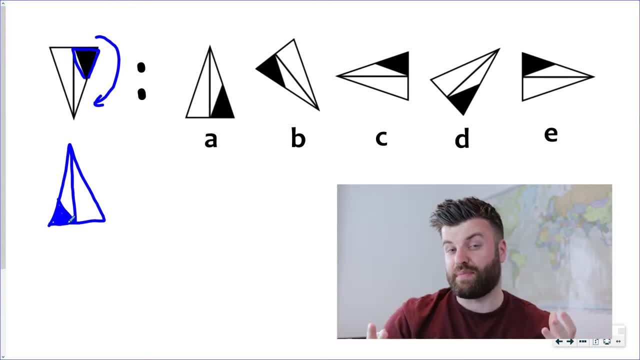 the right, having two angles to work from, where you know the shape looks like, that might just help you with deduction, getting rid of those answers that are wrong and actually finding the right one. so let's use these shapes- now we've got on the left- to try and find our answer. on the right, we can. 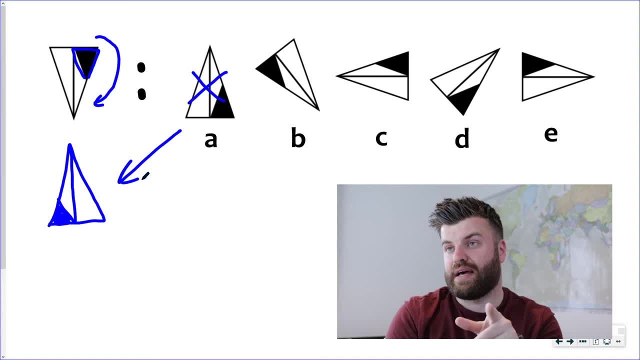 see straight away, it's not a, because that does not match the rotation we've just made ourself b. can that work? well, if we take a look at the original shape and rotate it slightly anti-clockwise, you can see that the blue, the black shaded bit should be there. it's not, so it's not being. 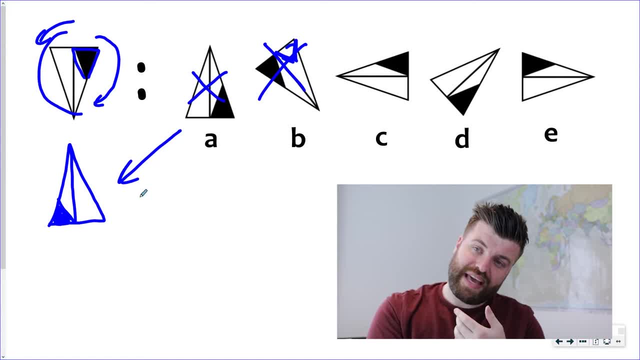 looking at C again. look at our base. down here the black shading is on the left now because we've rotated it. if our base is here, the black shading should be on the left and it's not. so it's not C, and slowly, by deduction, we're down to two already. so is it D or is it a? now let's. 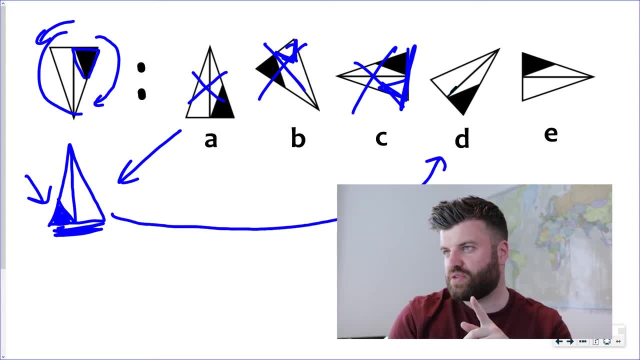 compare D to this one. at the bottom, the shadings on the right. our shading should be on the left when it's rotated. so it's not D and we're left with a. we're gonna cross our fingers and hope that's the answer. we'll put e down, but we'll just make sure now, if this is our base is the black. 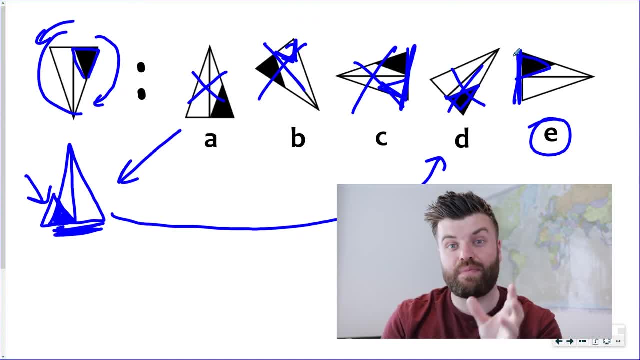 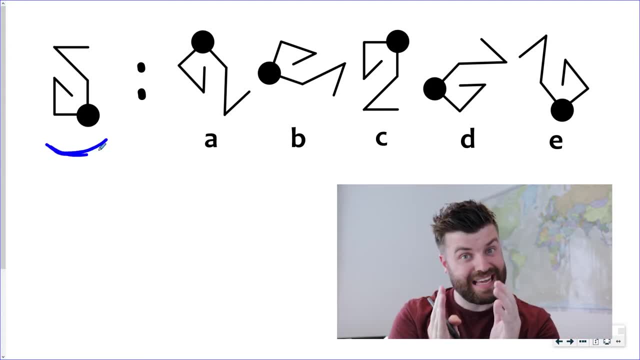 shading on the left. yes, it is, it matches up. we'll put a and we can move on to the next question. so on the screen now, we've given you a shape on the left hand side and we want you to have a go matching up with one of the five shapes on the right. now, before you do that, let's just have a. 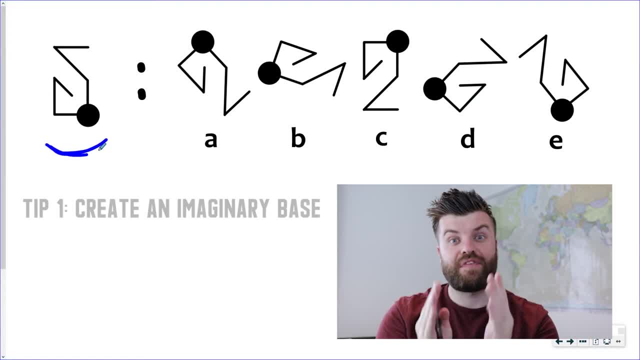 quick recap of those techniques we talked about. try and find a base for your shape and then look at the features and how they relate to that base. does it move to the right? is there a circle to the left? is there some shading at the top? those can help. 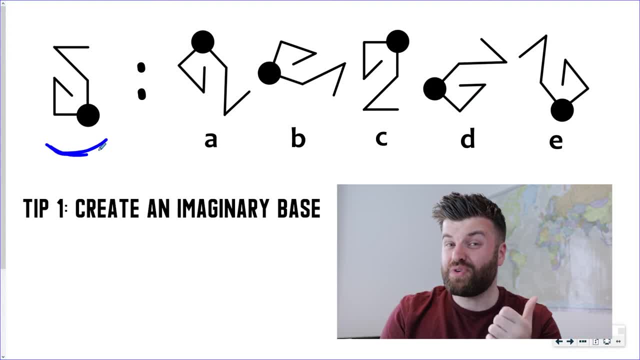 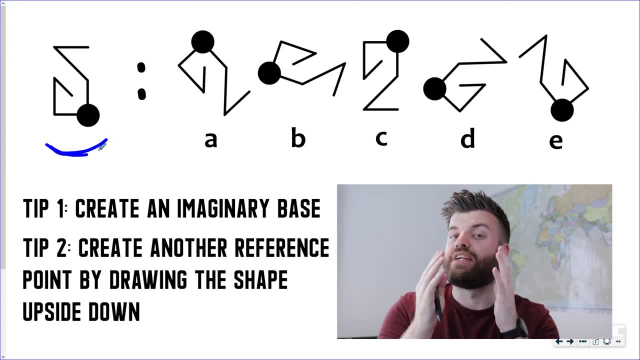 you to draw comparisons to the shapes you're trying to find and also if you can just rotate that shape in your mind's eye, practice moving it without actually moving your paper, and draw a shape that's 180 degrees rotated. you have two reference points now to work from, which can 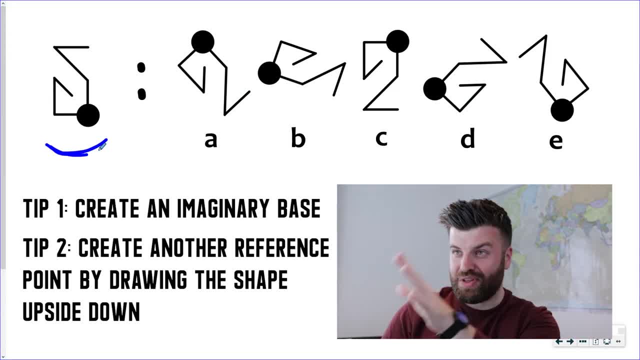 really help you find the right shape. so have a look at the one on the on the screen. I want you to try and find an answer and if you get one, if you think you've found the shape which is exactly the same as the one on the left. but